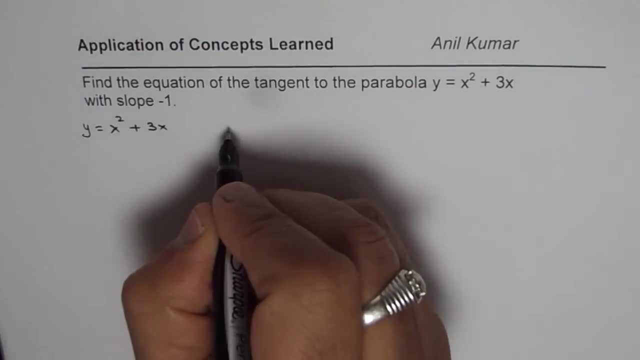 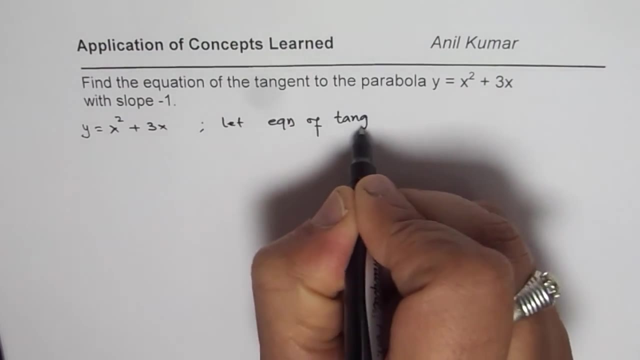 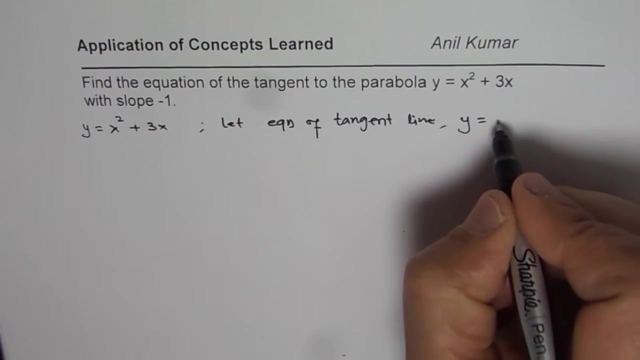 So let us say equation of tangent line is: so let us say: let equation of tangent p- y equals to slope, is minus 1, so let minus x plus p, right? So basically we need to find b to get the answer right. 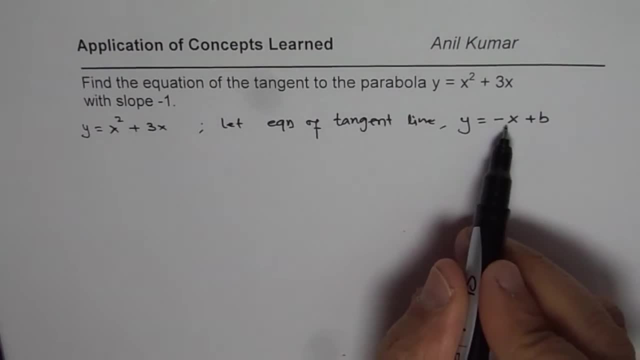 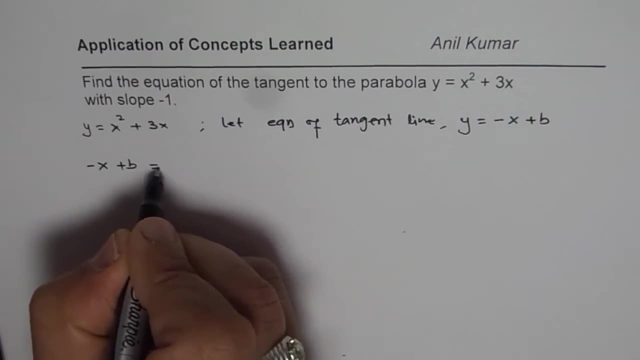 So what we will do is we will replace y with minus x plus p in this equation and then solve the two equations. So what we have here is minus x plus b equals to x square plus 3x. bring the terms together: we get x square plus 3x plus x minus p equals to 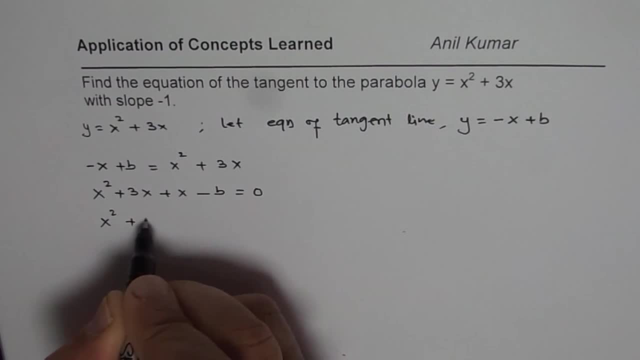 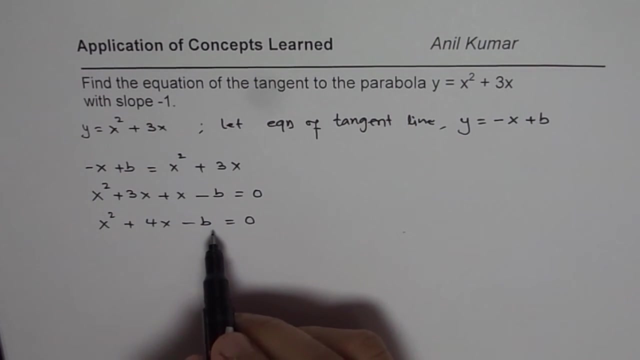 0, which is x square plus 4x minus p, equals to 0. right now, that is the equation which needs to be solved and we need. we can use quadratic formula to find the value of x. that is one way, but what we need here is to find the value of b. right, that is what we need. 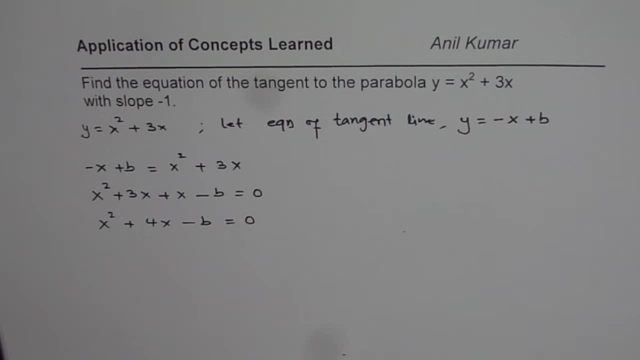 so how do we do this kind of equation? well, if we are looking for a tangent, then we have only one solution to this equation. that means, if you are looking for a tangent, so for tangent, tangent, so for tangent, so for tangent. there has to be just one solution, is it ok? so how do you get one solution for a quadratic? 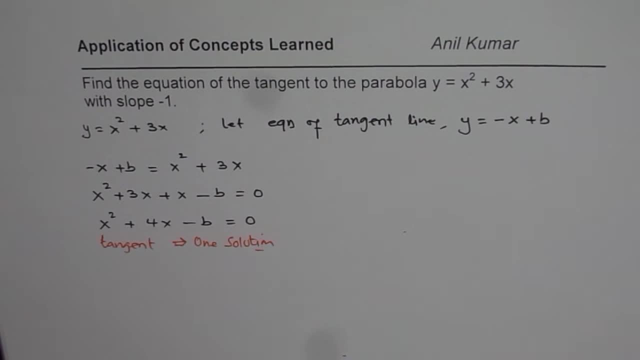 equation. you get one solution for a quadratic equation in general if b square minus 4ac is equals to 0, right? so that is the concept which we are going to use in this particular equation. when i say b square minus 4ac, i am looking at the equation as ax square. 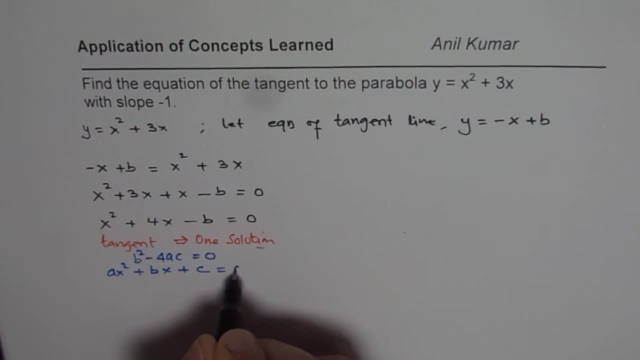 plus bx plus c right equals to 0. so that is the equation which i am looking at, right? so you should not confuse with these two b's together, right? so? so this is, this is what we are going to apply, right? so in our equation, what is a, what is b and what is c? in our equation, we have a as equals to 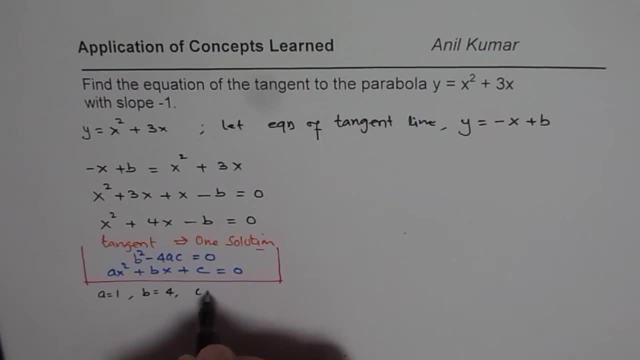 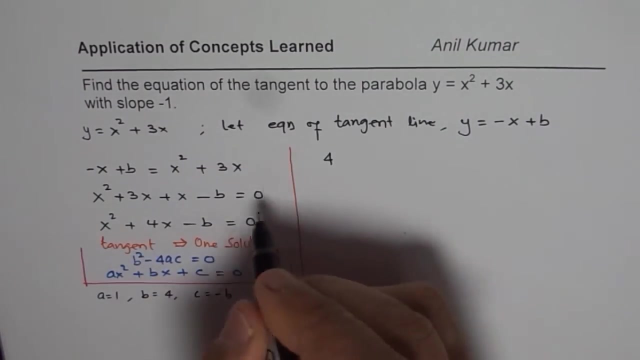 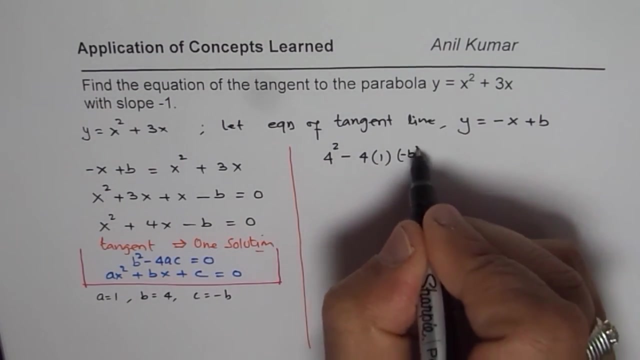 1, b as equals to 4 and c as equals to minus b. do you get the idea? right now we will find the value of b by equating b square minus 4ac as equals to 0. so that means if i say b square minus 4ac, that means 4 is my b. so 4 square minus 4 times a is 1 and c is minus b. that should. 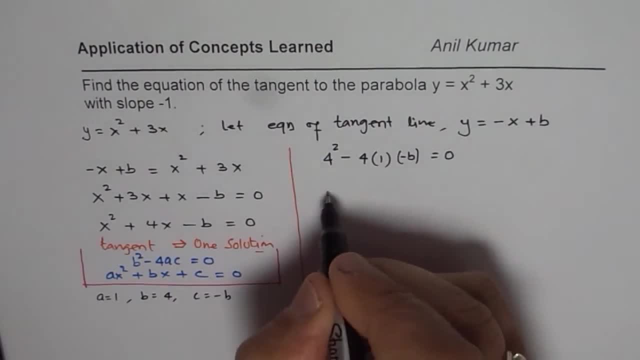 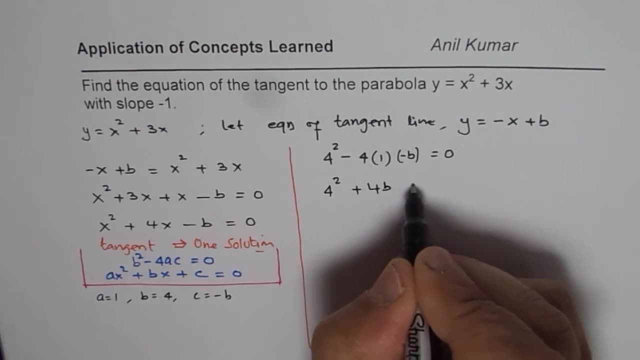 be equal to 0. you get the idea now we can solve for it. so we have 4 square minus and minus becomes plus. we get plus 4, b equals to 0. we can solve for b now. so well, you could take 4 common and you get 4 plus b equals to 0, so that 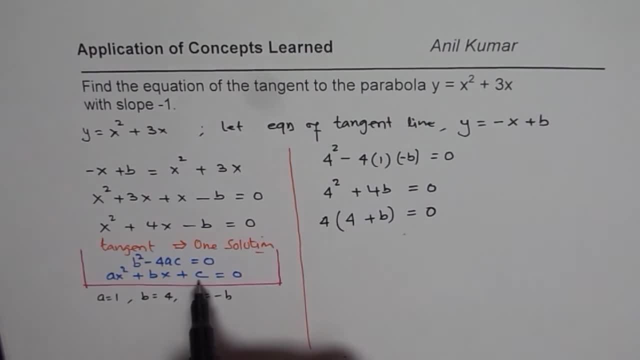 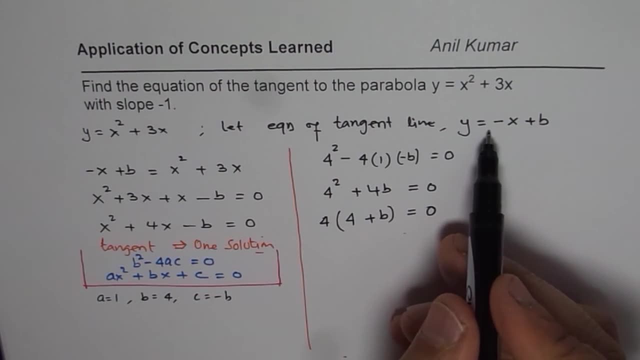 is a factoring technique which you know about right, and this is the quadratic number of roots you have learned correct. now this is solving linear systems with quadratic systems. so these are so many principles which we are combining together. now, when will this be? 0, this will be. 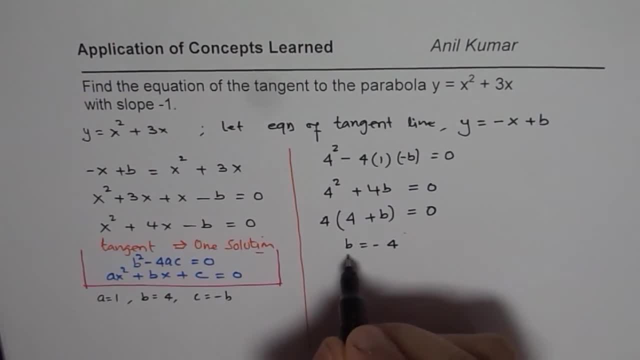 0 for b equals to minus 4, right? so that is the equation which we are going to apply right now. that is the value of b. once you know what b is, you can find the equation of the tangent line right. so therefore, the equation of tangent line is: y equals to minus x, minus 4. you get the idea. 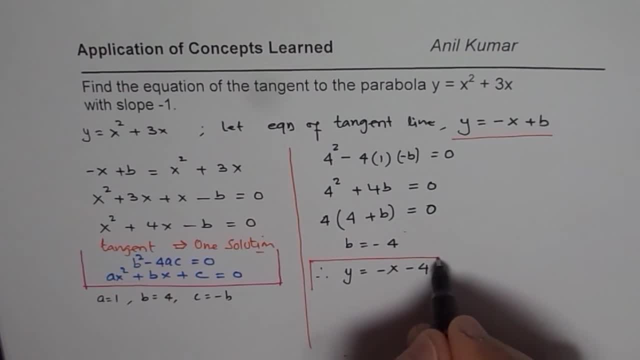 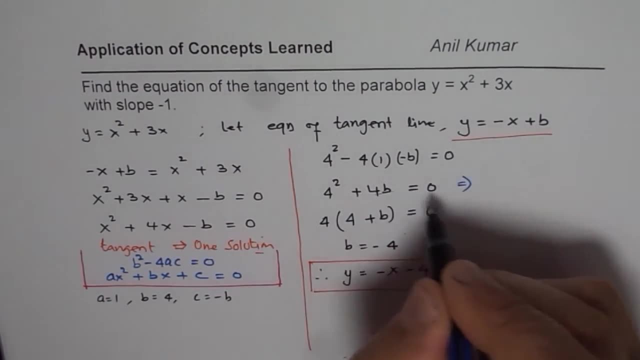 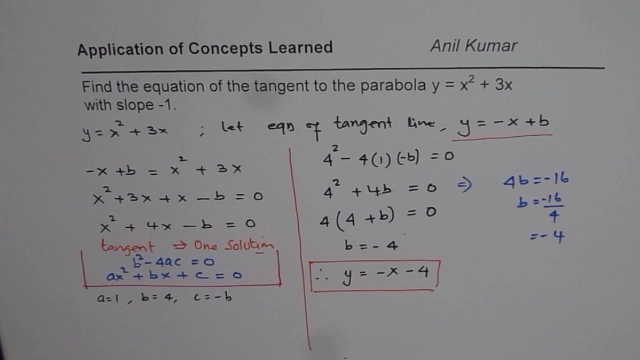 right. so that is how you can actually solve such questions. all right, you could always from here also solve directly, saying that 4b is equals to 16 and b is equals to 16. i'm minus b is minus 16 by 4, which is minus 4. that's fine, also right, so either way. so what we have. 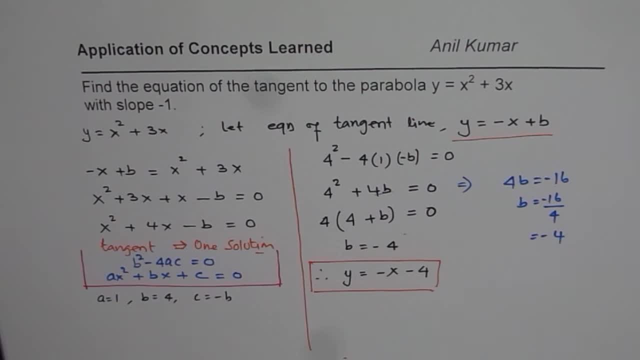 learned here is that how to solve linear systems, how to ensure that we have only one solution for the given linear system, and how to understand the situation and apply different techniques. i hope that helps. thank you and all the best you.